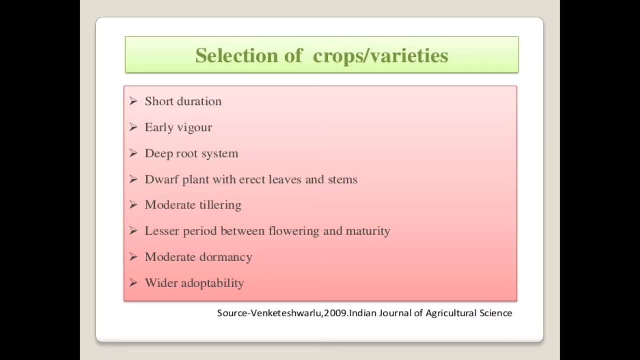 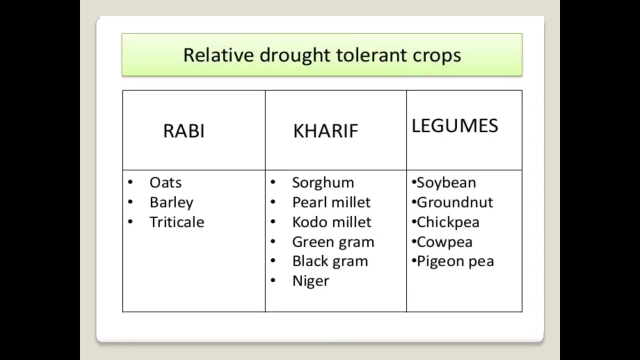 Then the selected crops or the varieties should have the moderate dormancy And the selected crop or variety. they should be widely adopted by the condition of that locality. Then there are some relative drought tolerant crops which are selected in the different seasons, For example in Kharib season. 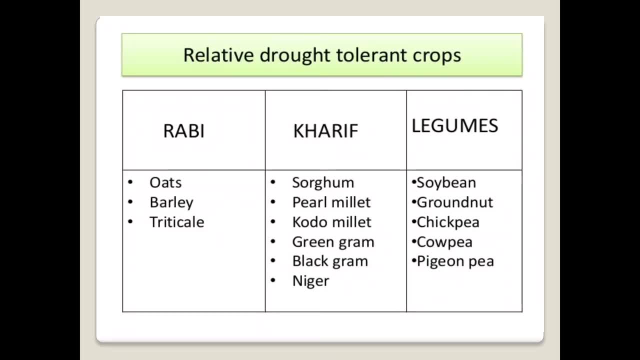 The crops like the Sorghum, Pearl Millet, Kodo Millet, Green Gram, Black Gram and Niger, which are suggested. Then, in case of the Rabi crops, The crop selected are Oat Barley and the Feet that means the triticale. 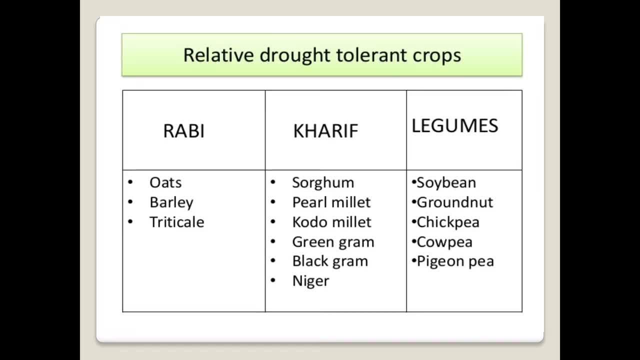 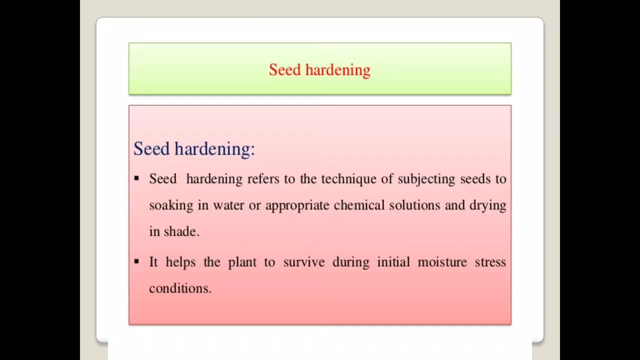 Then, under the legume crop here, some crops which are selected to mitigate the drought condition, That is Soyabean, Walnut, Chickpea, Cowpea and Pigeon Pea. Then the second crop management practice, that is the seed hardening. 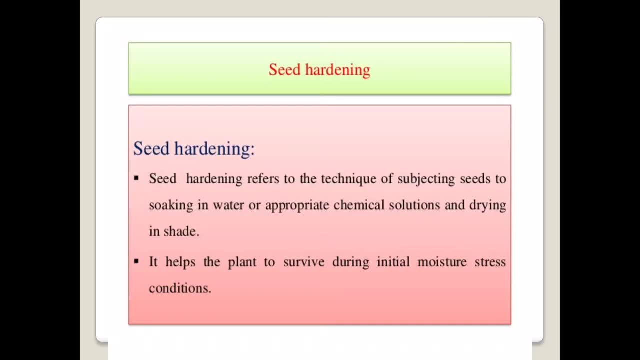 Then what is the seed hardening? So the seed hardening is defined as it refers to the technique of subjecting, Subjecting the seeds to soaking in a water or the appropriate chemical solution and they are dry in a shade. That means known as the seed hardening. 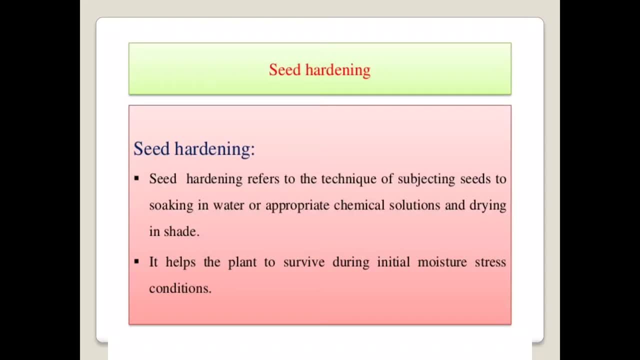 Simply The techniques of the seed hardening. that involves the whatever the seeds which are selected, The selected seeds, they are soaked in a water or the another solutions of the chemical, and after that the seeds which are dry in a shade. Particularly this seed hardening that helps the plant to survive during the initial moisture stress condition. that means 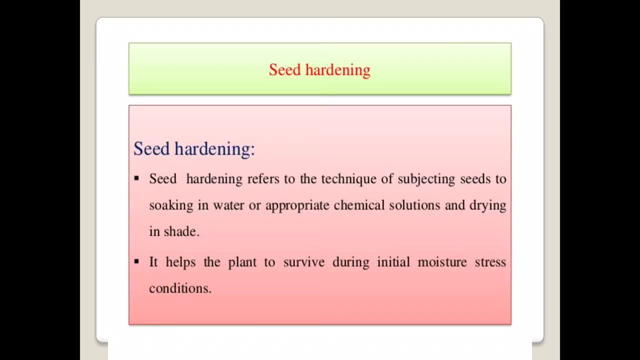 By the application of the seed Seed hardening. that seed hardening that helps to survive the crops during the initial moisture stress condition. That means during the initial growth stages of the crop. So this is also the one of the important technique for the mitigation of the drought under the rainfall condition. 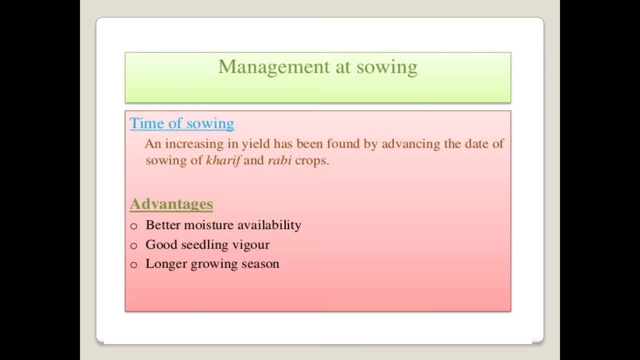 Then, what are the different management practices which are followed for the mitigation of the drought? that management practices? which management practices? It involves the time of sowing, So the time of sowing that also plays a very important role in increasing the yield as well as the mitigation of the drought in a rain fed condition. 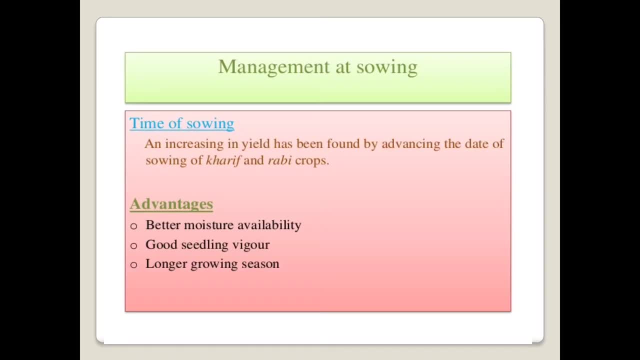 An increasing yield has been found by advancing the date of sowing in a Kharib, as well as the rubbish crop Means the time of sowing. that plays very important role when we are adopting the timely sowing operation in case of the Kharib crop. 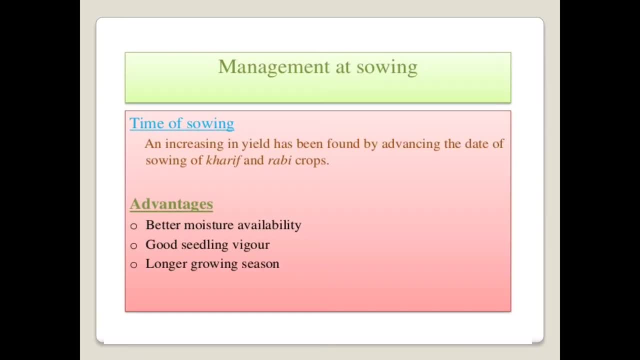 As well as the rubbish crop that helps to increasing the yield drastically. Then what is the advantages of the time of sowing? that means when the sowing, which is carried out in a time. So there are three main advantages of the timely sowing of the crop. 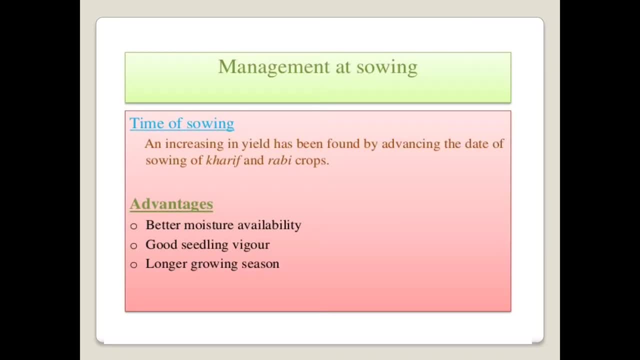 First one, that is, the made better moisture availability. when we have to, we have carried out the sowing operation timely and in that condition, The whatever The moisture which is which is available that is used efficiently and in that case the germination of crop is takes place in a better way. 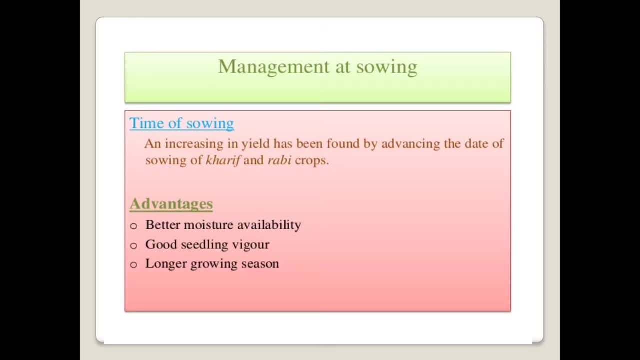 Then it also gives the good seedling figure. That means during the initial growth stages, the seedling, they are well developed. Then, third one, that is the longer growing season. when the sowing operation that is carried out in time, in that condition, the long, longer growing season. 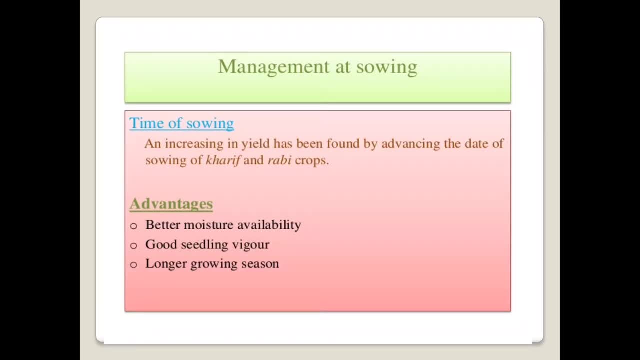 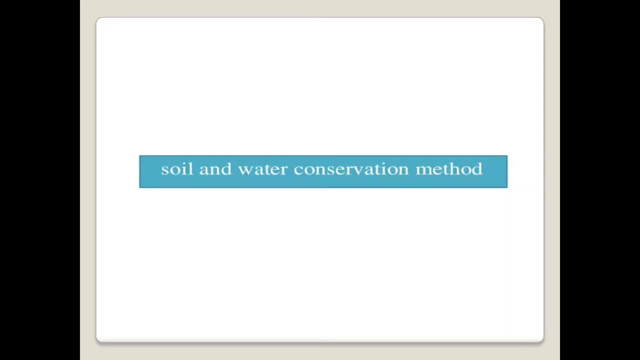 That is available for the growth and development of the crop. Then there are some soil and water conservation methods which are used to mitigate the drought condition in a rain fed area. That means the various soil conservation as well as the water conservation methods which are applied to reduce or to minimize the drought under the rain fed condition. 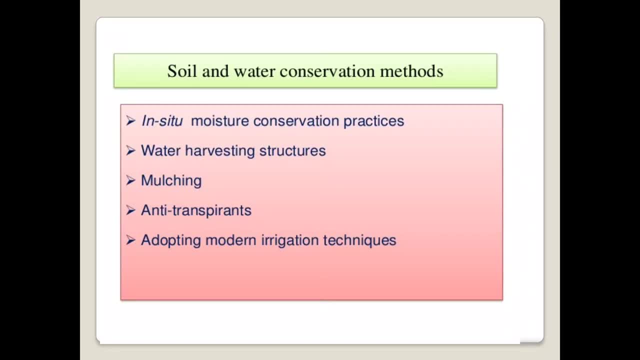 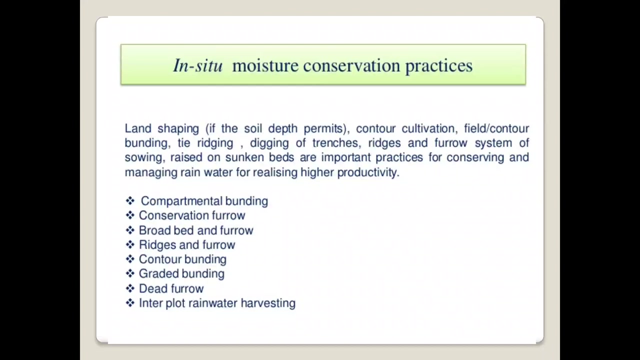 So this soil and water conservation methods, that involves the in situ moisture conservation Practices, then water harvesting structures, Then the application of the mulches, then use of the various anti-transparent and the adopting the modern irrigation techniques. So these are the various soil and water conservation methods which are used to mitigate the drought condition, in that the first and most important practice. 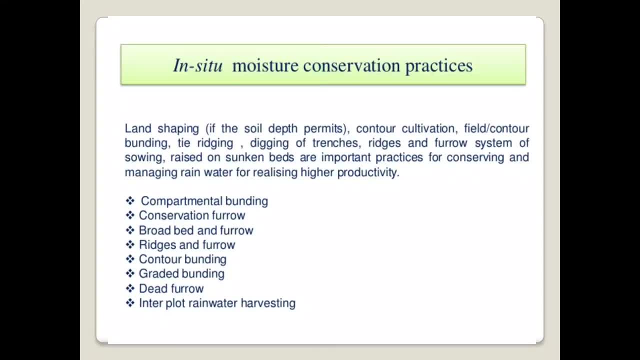 That is, the in situ moisture moisture conservation practices. It involves the land shaping, then country cultivation field For the contour banding, tie ridging, then digging of the trenches, ridges and furrow. system of sowing, Then raised on a sunken beds, are important practices for the conserving and managing the rain water, for realizing the, for realizing the higher productivity. 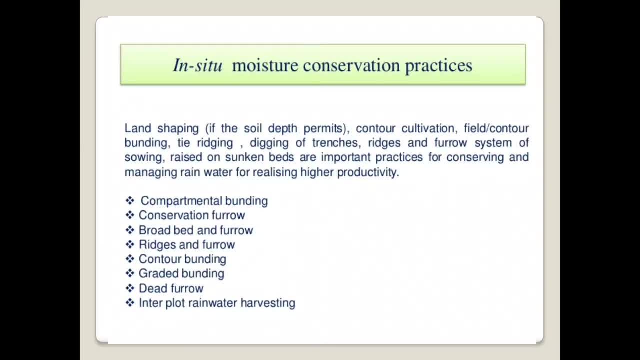 Here some in situ soil moisture conservation practices, which includes the compartmental banding, then conservation furrow, then the construction of the broad bed and furrow, then ridges and furrow, Then next one, that is, the contour banding, graded banding, then dead furrow, and inter plot rain water harvesting. 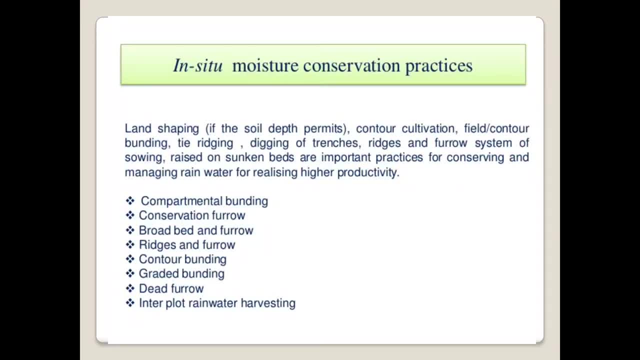 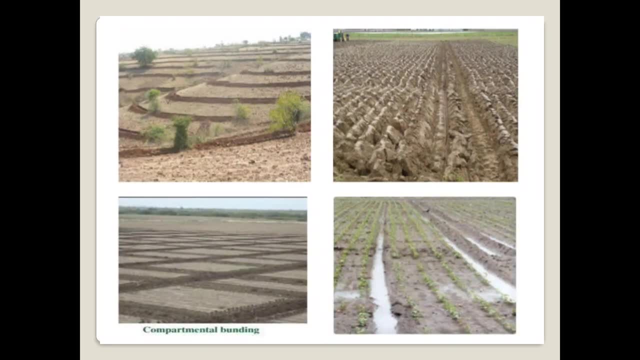 So these are the various techniques which are included under the in situ moisture conservation practices. In this figure they show. this figure shows the various in situ soil moisture conservation practices, For example compartmental banding, then Dead furrow, back furrow. so this figure, that showing the various in situ soil moisture conservation practices. 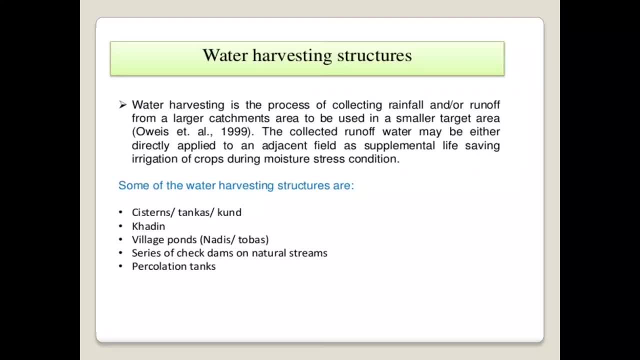 And that practices, which helps to store the maximum water into the soil, and it also helps to mitigate the drought condition or to minimize the drought condition under the rain fed situation. Then the next one, that is, the water harvesting structure. So, firstly, What is the water harvesting? we should know the definition or the concept of the water harvesting. 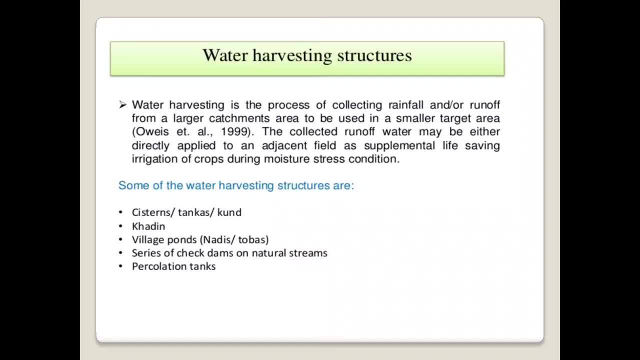 So the water harvesting is the process of collecting rain water, rainfall or the runoff from a longer catchment area That is to be used in a smaller target area. That means whatever the excess water after the receiving of rainfall that is collected and stored from the larger catchment area. 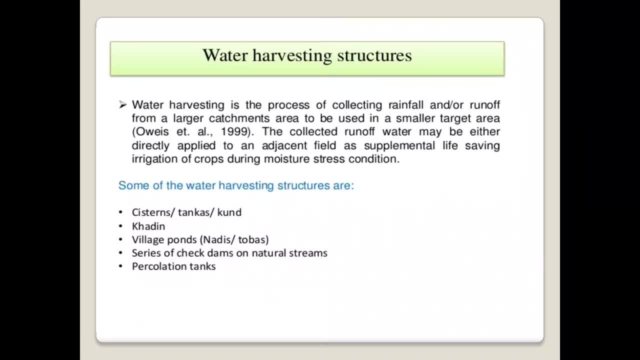 And that stored water that is useful for the small area in future for the cultivation Of the various crop. The collected runoff water that may be either directly applied to the adjacent field as a supplemental life saving irrigation of crops during the moisture, During the moisture stress condition. that means, whatever the harvested water is there and the collected runoff water is there, 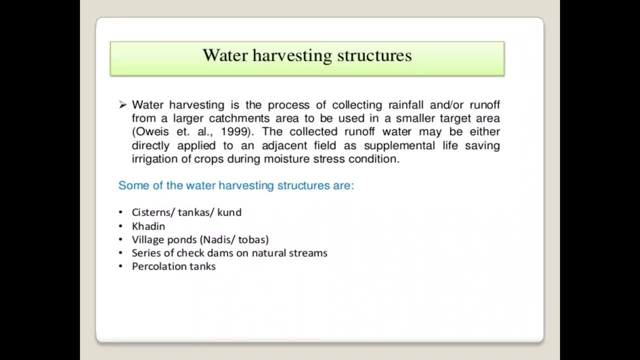 That is in. first. The collected runoff water Is Used For the two purpose. Firstly they are directly applied to the field as a supplemental irrigation, And again it is also used during the moisture stress condition. Then there are some water harvesting structures. are there? 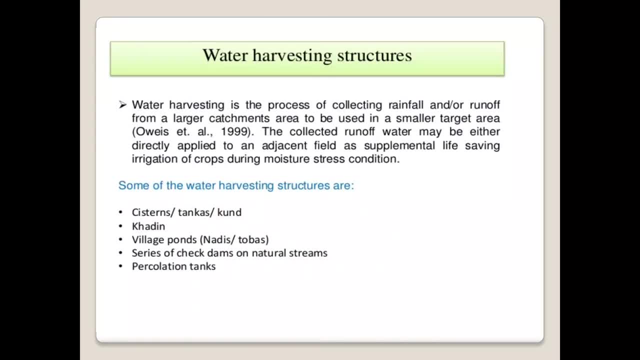 These are the systems That is also known as the tankas or the kunda. Then second one is the khadi, Third one is the village pond, Next one is the series of check dams on the natural stream And last one is the percolation tanks. 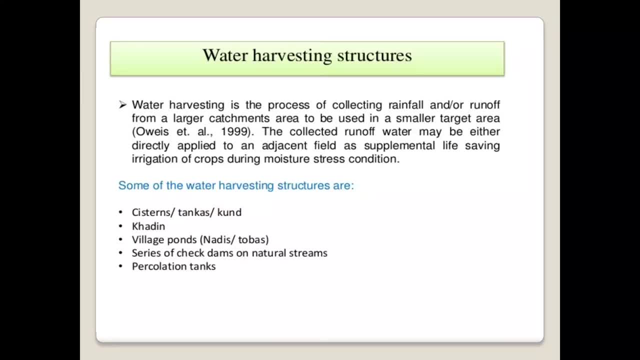 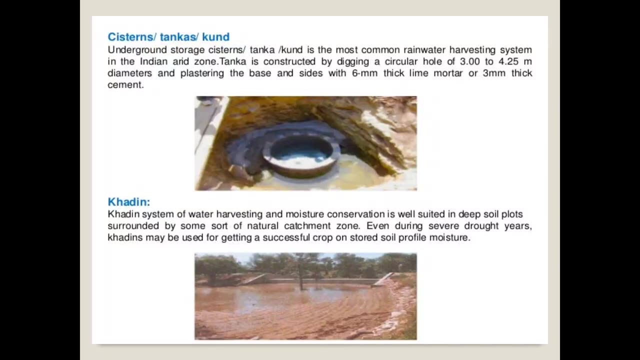 So these are the various water harvesting structure. that means whatever the water that is collected from the runoff, water that is stored in the water harvesting structure, Then the first water harvesting structure, that is, the cisterns or the tanka, or it is also known as the kunda. 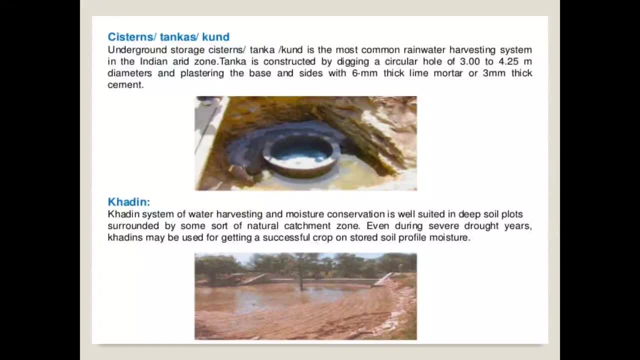 So this is the first water harvesting structure. Under this, the underground storage cistern tanka, or kunda, is the most common rainwater harvesting structure. That is the most common rainwater harvesting system That is particularly used in the Indian arid zone. 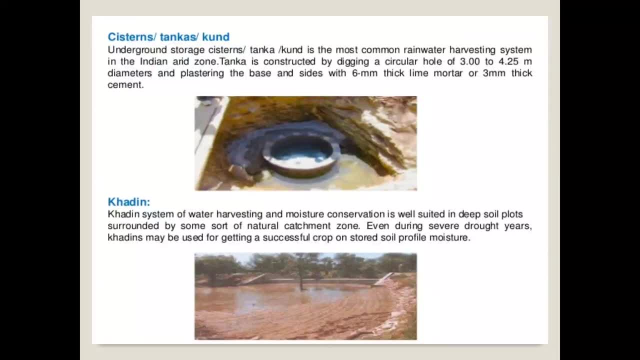 Means those area which receiving the rainfall of a very less amount. Then this tanka is constructed by the digging a circular hole of 3 to 4.25 meter diameter. Then the cisterns, they are constructed in the earth surface Which having the dimension, that means which having the circular hole of 3 to 4.25 meter diameter. 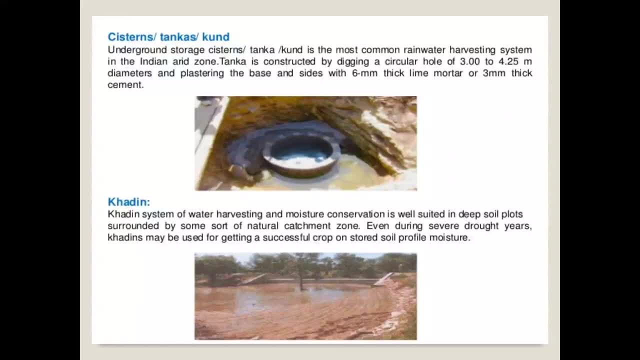 And they are plastered, the base and side, with the 6 millimeter thick lime mortar or 3 millimeter thick cement. So this is the first water harvesting structure, that is, the cistern tanka, or it is also known as the kunda. 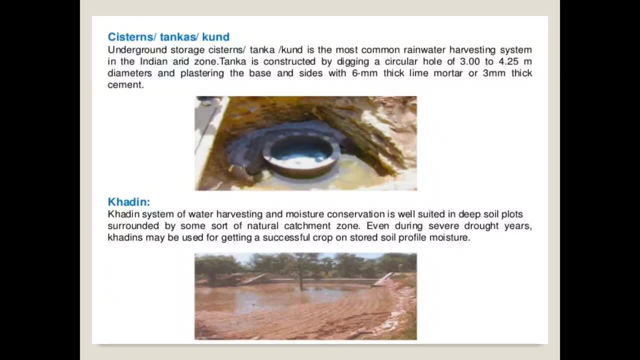 Then next one is the khadi. So this khadi system of water harvesting and the moisture conservation That is particularly suited for the soil plot that is surrounded by some of the natural catchment zone. Even during the severe drought year the khadi may be used for getting a successful crop on a stored soil profile moisture. 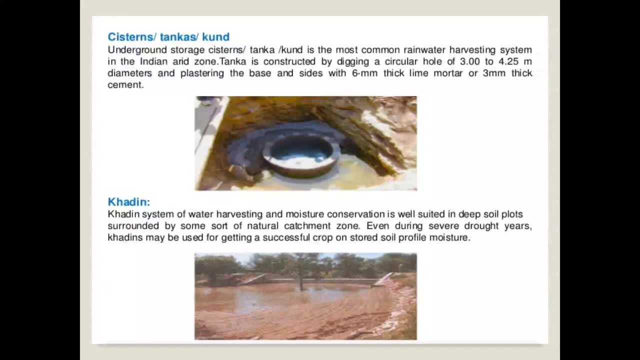 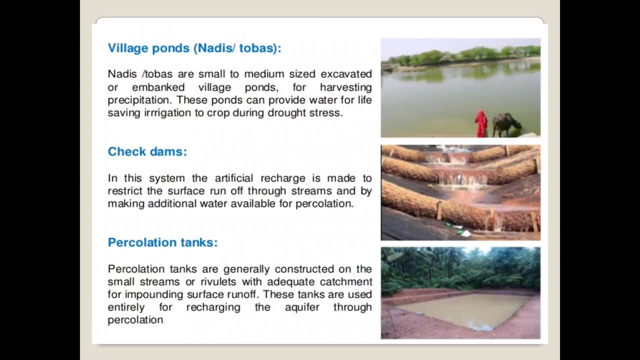 So this khadi system of the water harvesting that is useful during the severe drought year And they are useful for getting the successful crop production On the stored soil profile moisture. So this is the second water harvesting structure Which is used mostly during the drought years. 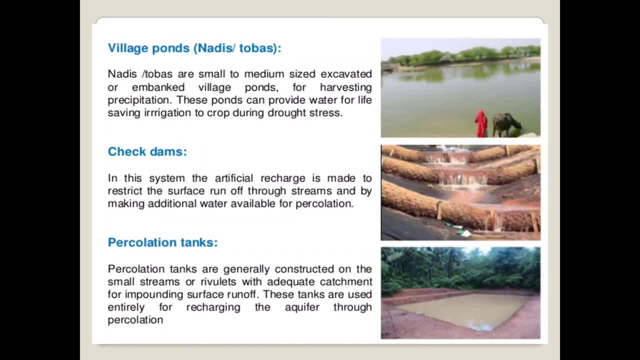 Then next one is the village pond That is also known as the nadis or tobas, Then nadis. they are the small to medium sized excavated or the embanked village ponds. They are used for the harvesting of the precipitation, These ponds that can provide the water for the life saving irrigation to crop during the drought stress condition. 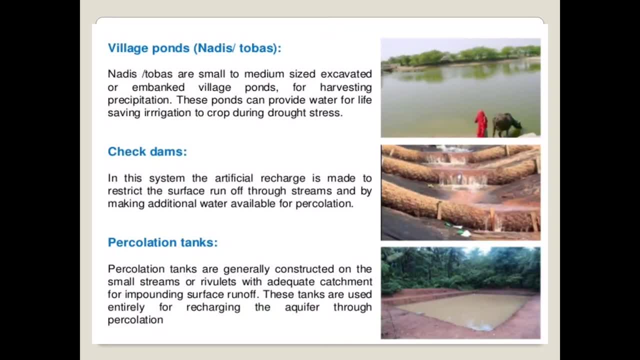 Whatever the water that is stored in this village pond that is used for the life saving irrigation, That means whatever the stored water is there and that stored water which is used for saving the life of crop And which is given to supplement the irrigation. for that purpose, this stored water is useful. 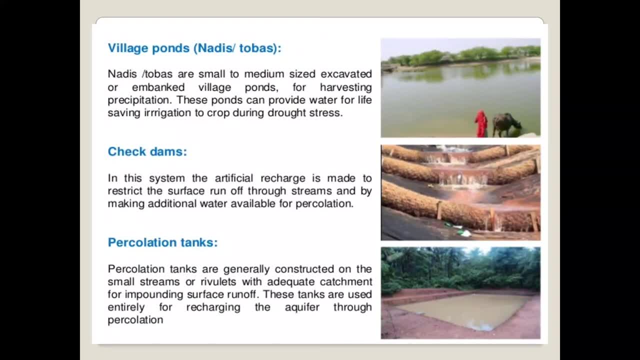 Then Next water storage structure, that is, the check dam In this system, the artificial recharge that is made to restrict the surface runoff through the stream And by making the additional water available for the percolation, So this check dam. they are the artificially constructed obstacle to the flowing water. 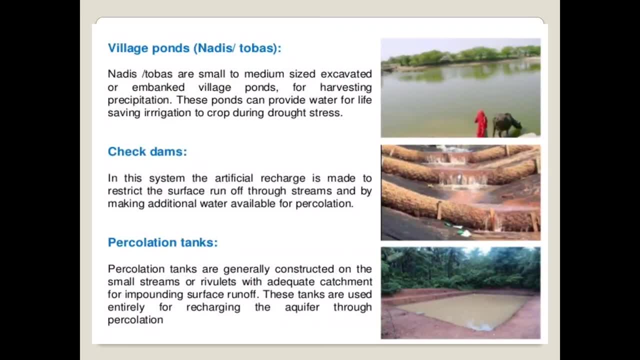 And the excess water that is allowed to flow from that structure that is known as the check dam. Then next one is the percolation tank. So this percolation tanks, they are generally constructed on the small stream With the adequate catchment for impounding the surface runoff. 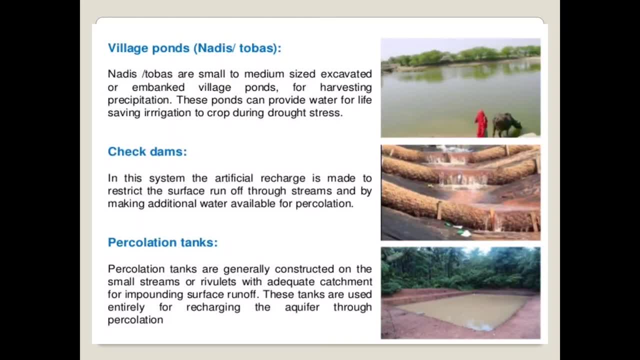 That means this percolation tanks which are constructed in a small stream, That means where the small flow of water is there And that area that should also having the adequate catchment area for collection of the surface runoff water. Then this tanks are used entirely for recharging the aquifer through the percolation. 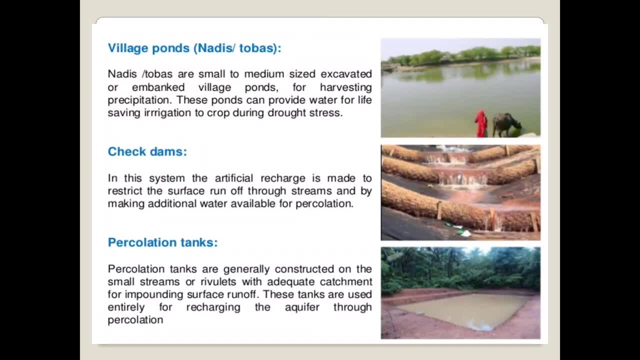 So this is the fourth water harvesting structure, Particularly useful in the rural area for the storage of the runoff water And again, it is useful for the cultivation of crop, As the water which is stored in this percolation tank, which is used for the life saving irrigation to the crop, 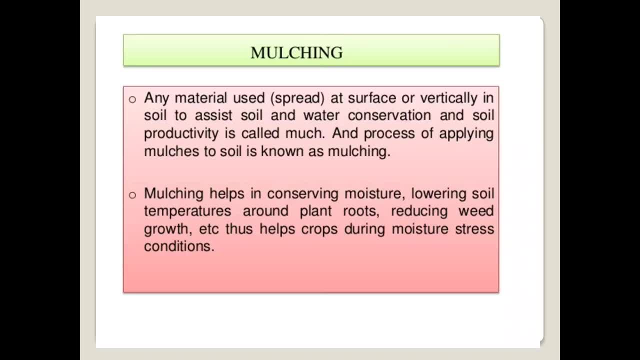 Then next important practice which is used to mitigate the drought. That means this is also used to minimize the drought condition in the rainfall situation. That is the mulching. So we should know the definition as well as the concept of mulching. So firstly, we will discuss about the definition of mulching. 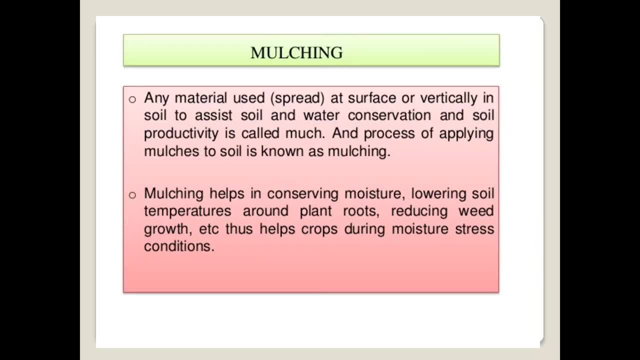 So the mulching is defined as the. any material which is used at the surface or vertically in soil to assist the soil and water conservation And the soil productivity is called as the mulching. In simple way, the mulching or the mulching material, that is, the. it is the organic or inorganic substance or the material which is spread on the surface of soil to cover the soil surface in order to minimize the evaporation. 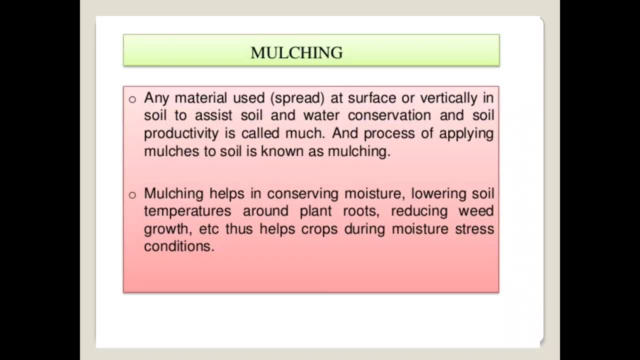 Then in maintaining the temperature of soil as well as the storage of the moisture into the soil- that is known as the mulching- And the process of application of mulches on the soil- that is known as the mulching. Then mulching helps in conservation of the moisture. 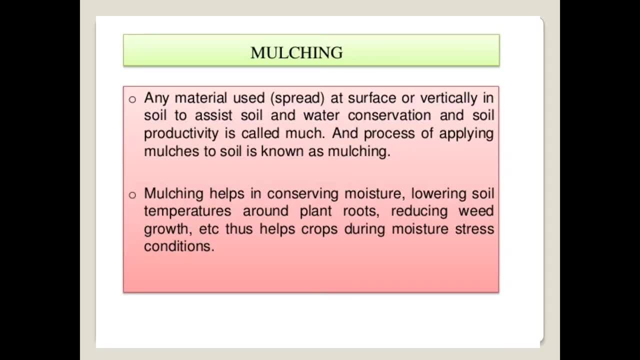 Then it also helps to lowering the soil temperature around the plant roots, Then it also helps to reduces the weed growth And it also helps crops during the moisture stress condition. That means the mulching having the several number of advantages as it helps to conserve the moisture. 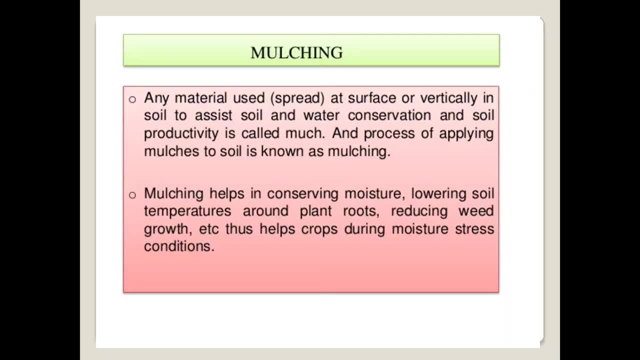 It lowers the soil temperature, Then it reduces the weed growth, Then it helps for the storage of moisture during the stress condition. Again, weed intensity is also reduces. that means the mulching which, having the several number of the advantages- Then there are different types of the mulches- are there: 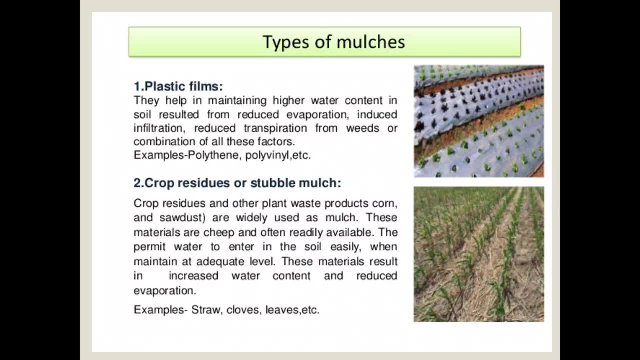 First one is the plastic film. They help in maintaining the higher water content in a soil resulted from the reduced evaporation, Then in increased infiltration reduces transpiration from the weeds or the combination of all this factor. So the first type of mulches, that is the plastic film. 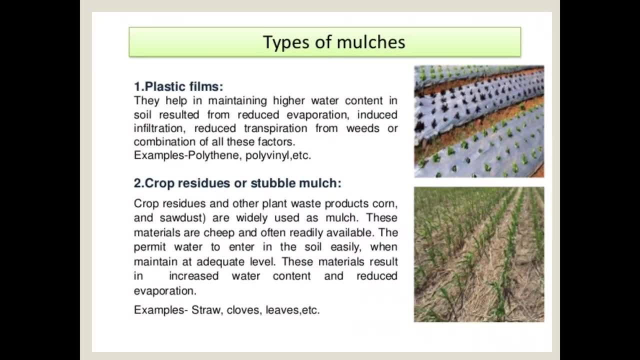 So this plastic film. they help to maintain the higher water content in soil. That means the maximum water that is stored into the soil. Then it also reduces the rate of evaporation, increases the infiltration rate of the water into the soil. Then it reduces the transpiration from the soil. 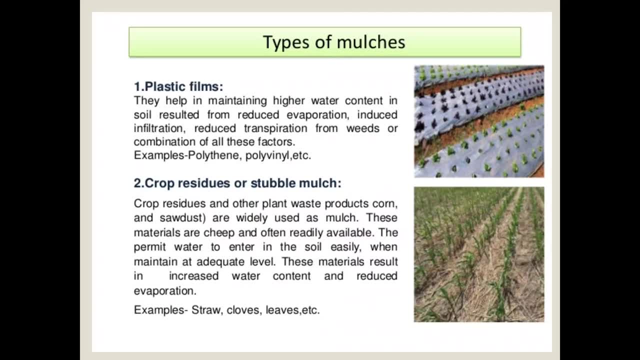 So these are the aerial parts of the plant. as well as the, they are useful in the all the combined factors. Then the examples of the plastic film. they are the polythene or the polyvinyl. These are the examples of the plastic film. 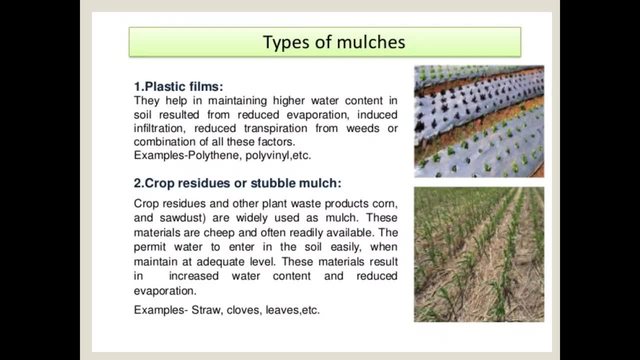 Then second mulch, second type of mulch, that is, the crop residue or the stubble mulch. So the crop residue and the other plant waste product, for example corn, as well as the sodas They are widely used as a mulch. That means whatever the waste material that is available on the farm that can be used as a crop residue or the stubble mulch. 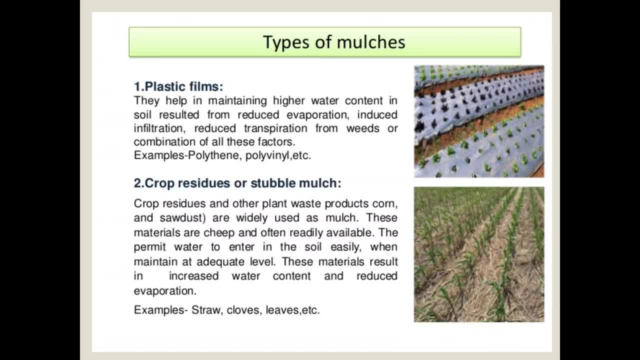 These materials are cheap and often easily available. That means this material which are used as a crop residue. they are very cheap, That means the cost required to purchase this material is very less and they are easily available. Then these material result in increased water content. 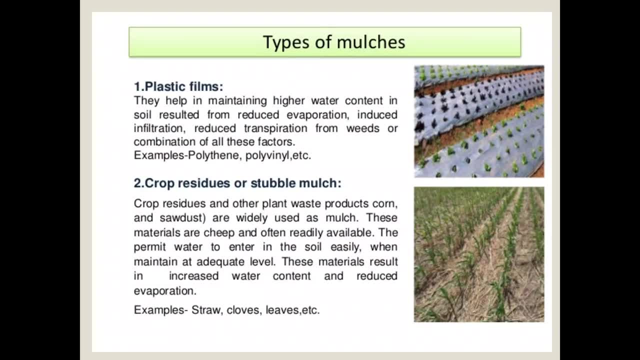 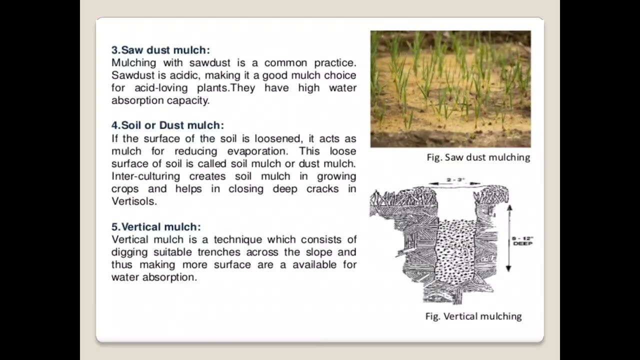 And reduces the evaporation, Then examples of the crop residues are the straw, then clothes, as well as the leaves. So this is the second type of the mulch, that is, the crop residue or the stubble mulch, The third type of the mulch, that is the sawdust mulch. 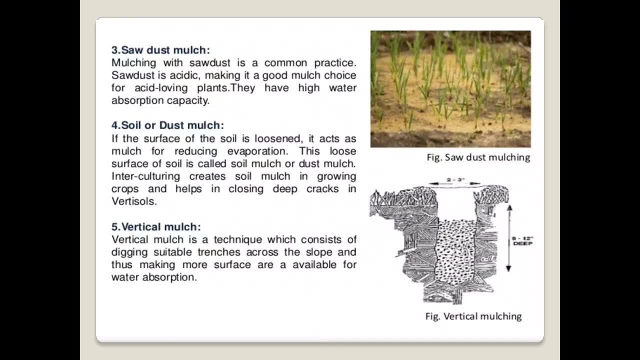 Mulching with the sawdust is a common practice. Particularly, the sawdust is acidic in nature, which help in making a good mulch choice for acid loving plants, Particularly the sawdust mulch which is used in the acid loving plant. then they have a high water absorption capacity. 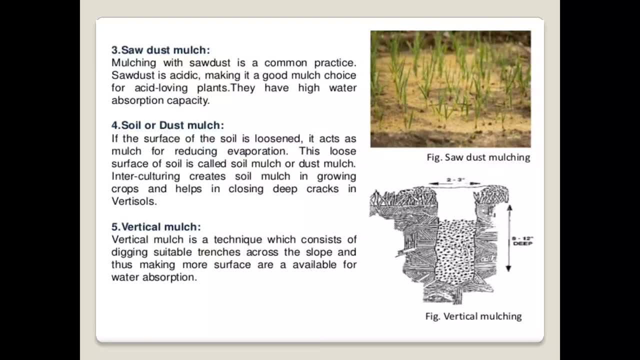 So the soil dust mulch. they absorb the higher water content than the other types of the mulches. The next one, that is the soil or the dust mulch. Then what is the soil mulch or the dust mulch? If the surface of the soil is loosen, it act as a mulch for reducing the evaporation. 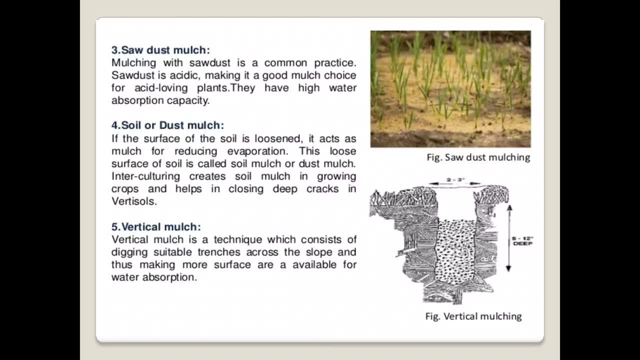 If the soil which is loosen through the air, If the soil is loosen through the, any practices which are carried out in the farm, And this loose soil which act as a dust mulch or the soil mulch. This loose surface is called as soil mulch or the dust mulch. 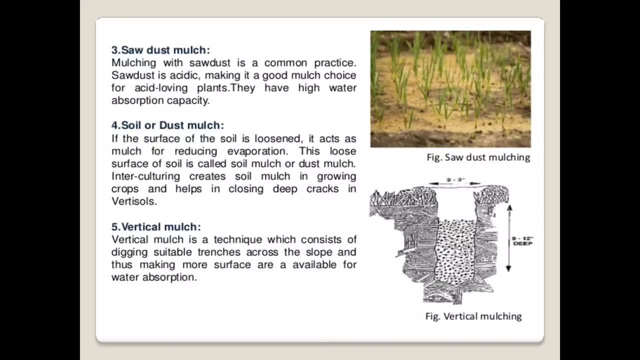 Then interculturing, that creates the soil mulch in growing crops and helps in closing the deep crack in a fertile soil. Then this soil mulch, or dust mulch, which having the important advantage as it helps in closing the deep crack which are formed in a fertile soil or in a black soil, 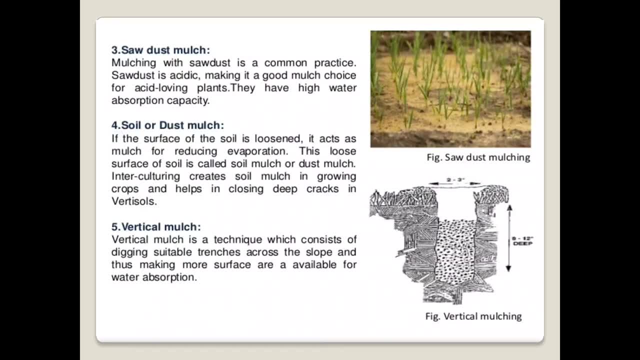 Then next type of mulch, that is, the vertical mulch. Then the vertical mulch is a technique which consist of digging a suitable trenches across the slope And thus making more surface are available for the water absorption. So this vertical mulch, that is the technique. 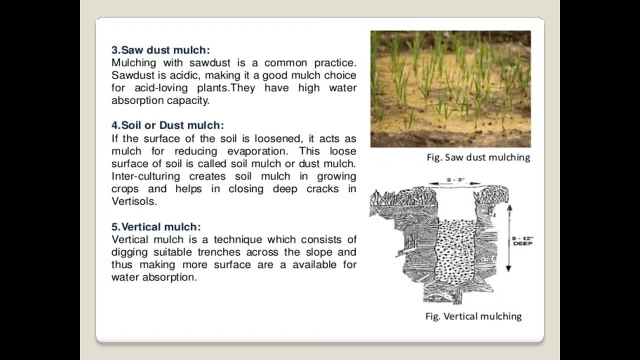 And it consist of the digging of the suitable trenches. And this trenches, which are digged across the slope of the land And due to that it makes the more surface which are available for the absorption of water. So this vertical mulch, which are available for the absorption of the water as well as the conservation of water, into 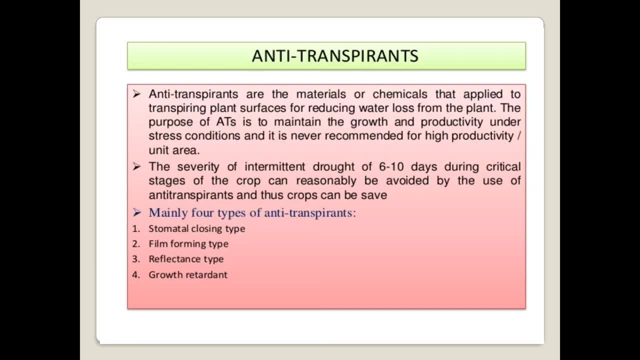 the soil. then the next important practice, which are used to mitigate the drought, that is the use of the anti-transpirant. so what is anti-transpirant? anti-transpirant: these are the chemicals of the material. they are applied to the transpiring plant surfaces, that is. 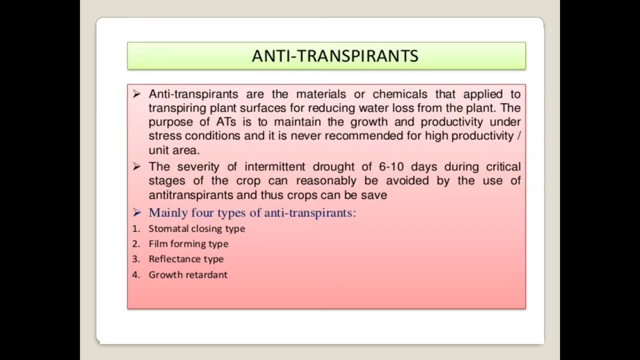 help for reducing the water loss from the plant. so particularly, whatever the chemicals or the any material that is that is applied on the plant surface- plant surfaces- in order to reduces the water loss from the aerial parts of the plant, that is known as the anti-transpirant. the purpose of 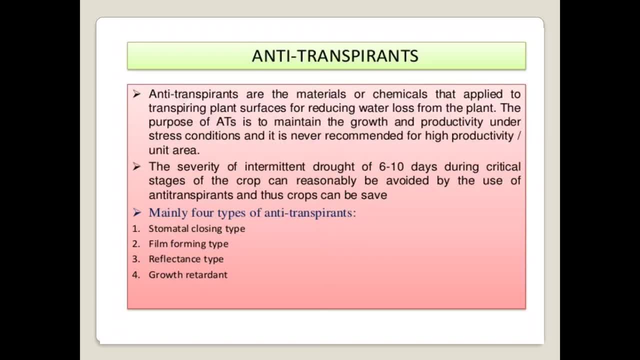 anti-transpirant is to maintain the growth and productivity under the stress condition. so what is the aim behind the application of anti-transpirant? anti-transpirant, that is to maintain the growth as well as the productivity of the crop under the stress condition, and it is never recommended for the high productivity per unit area that means. 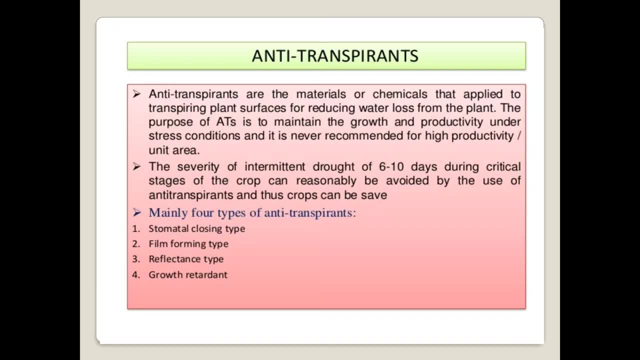 those area which having the high productivity per unit area. in that condition, the application of the anti-transpirant, which is not recommended. the severity of intermittent drought of six to ten years during the critical stages of crop can reasonably be avoided by the use of anti-transpirant, and thus crops can be saved. 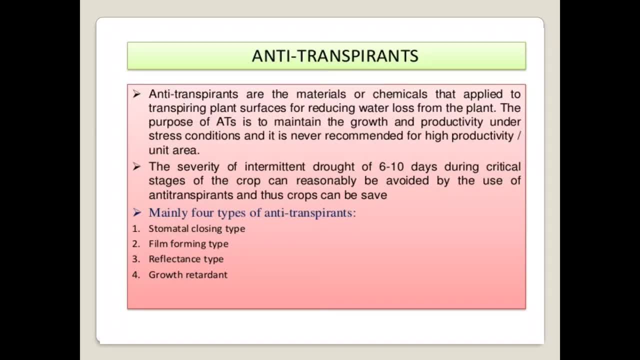 Then there are mainly four types of the anti-transpirants are there. first one is the stomata closing type of the anti-transpirant. Second one is the film forming type of the anti-transpirant. third one is the reflectance type of the anti-transpirant. 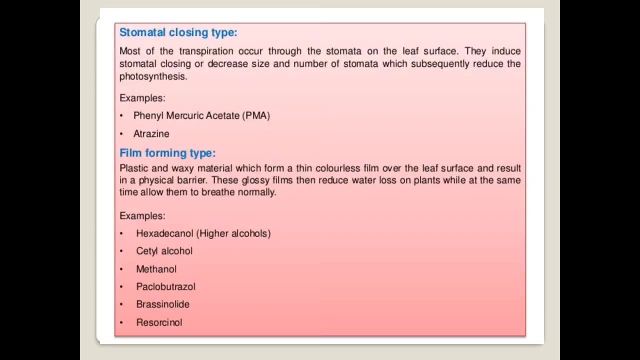 and fourth one is the growth retardant. So Firstly, first type of the anti-transpirant, that is the stomata closing type of the anti-transpirant. So Most of the transparency, most of the anti-transpirant there will be, cannot be, etc. etc. But for 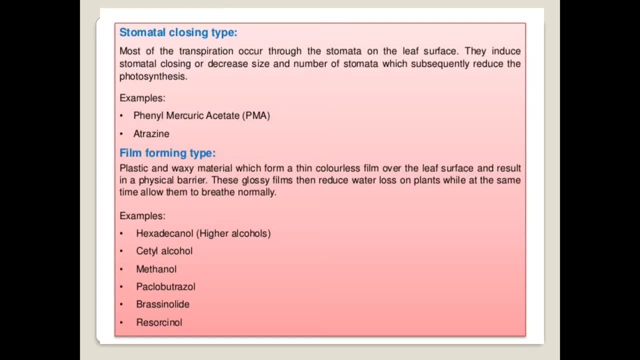 normal quote form. those are known categories that are ruined by Products or given a финal sayings. So you have transpiration which occurs through the stomata which are present on the leaf surfaces, so mostly the transpiration through the plant surfaces which is takes place by the stomata. 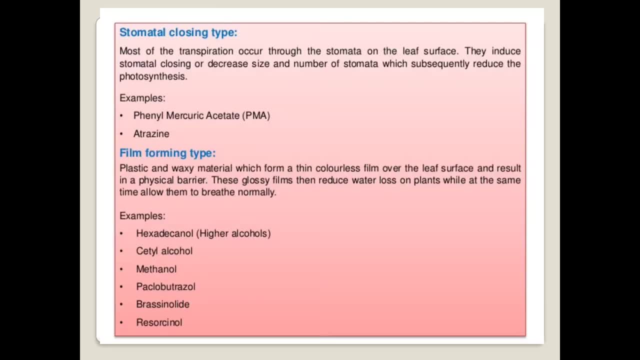 and these stomata which are present on the leaf surfaces of the plant. this stomata, they increases the stomata, sorry stomata closing type of the anti-transpirant: they increases the stomata closing or decreases the size as well as the number of stomata, which subsequently reduces the 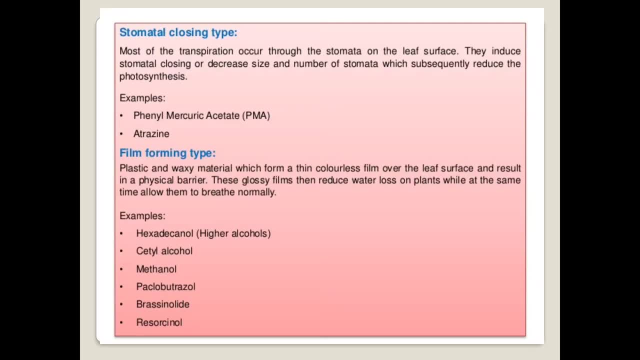 photosynthesis. then there are some examples of the stomata closing type of the anti-transpirant. they are phenylmercurycacetate, that means pma, and second one is the atrazine. these are the familiar examples of the stomata closing type of the anti-transpirant. then next one, that is the. 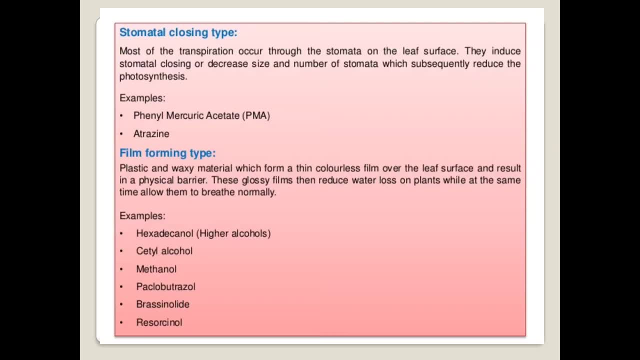 film forming type of the anti-transpirant, in that the plastic, plastic and waxy material which form a thin, colorless film over the lip surface and result in a physical barrier. so this film forming type of the anti-transpirant: they form a thin, colorless 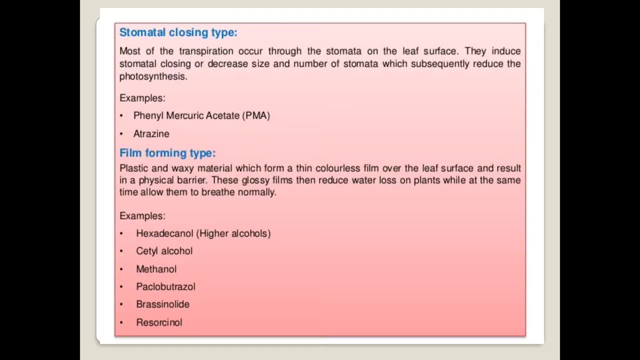 film over the lip surface and due to that they act as a physical, physical barrier in the process of the transpiration. then these glossy films: they introduces the water loss on the plant while at the same time they allow to breathe normally. so the the important function of this film, forming type of the anti-transpirant, the blue see film that are: 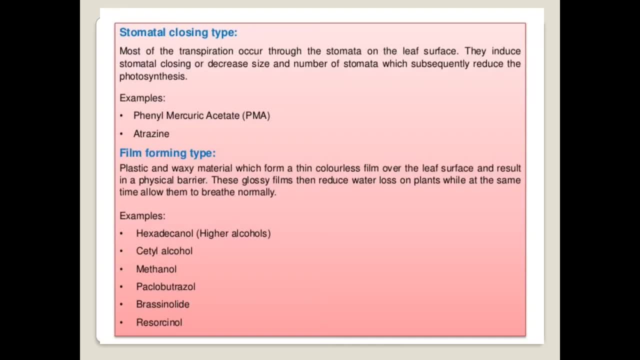 formed after the application of the film forming type of the anti-transpirant. they reduces the water loss through the plant and at that same time, they allow to breathe normally. that means the respiration which is takes place normally. then there are some examples of the film forming type. 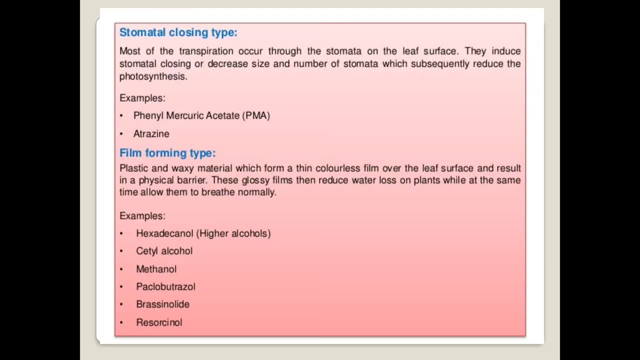 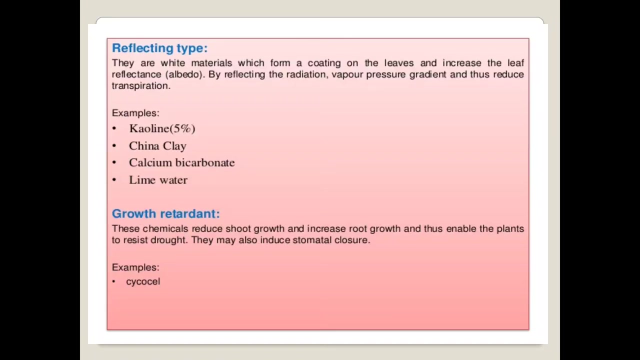 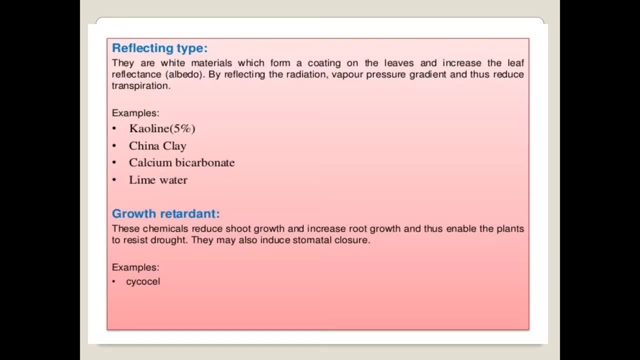 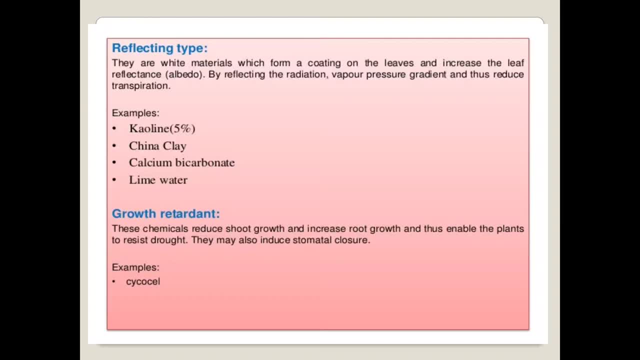 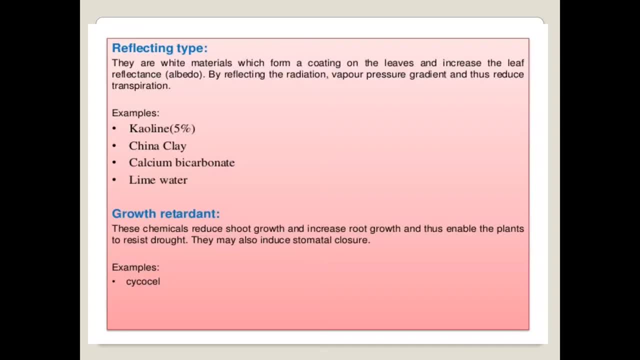 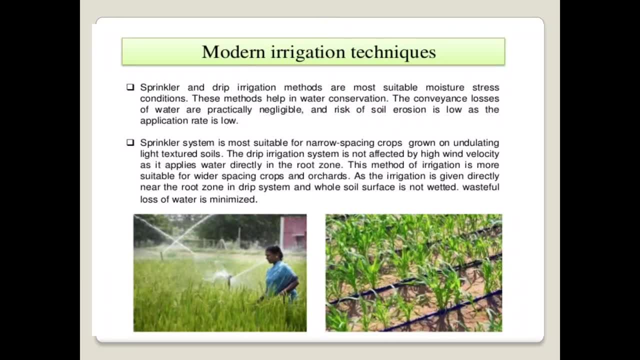 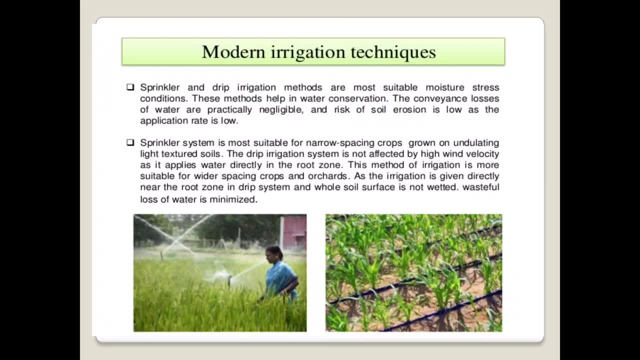 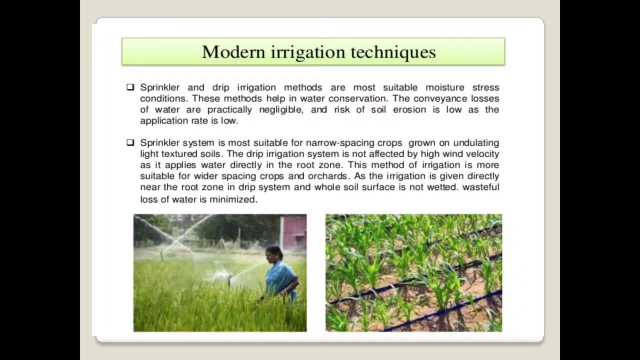 most suitable for the narrow spaced crops grown on the undulating light texture soil. then the drip irrigation system. that is not affected by the high wind velocity as it applies water directly into the root zone. that means when we are applying the water through the drip irrigation system and due 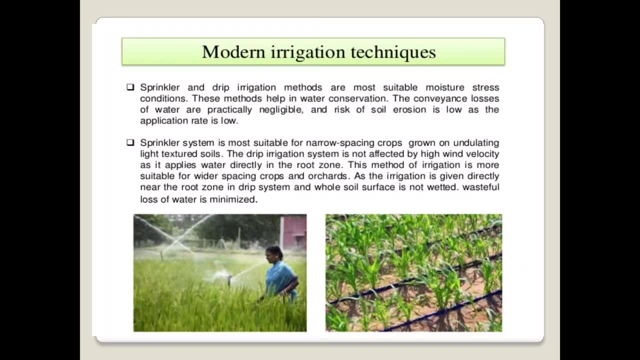 to that that is not affected by the high wind velocity because we are applying water directly into the root zone of the crop. this method of irrigation is more suitable for the wider spacing crops, as well as the orchard, the drip irrigation system that is mostly suitable for the those crop. 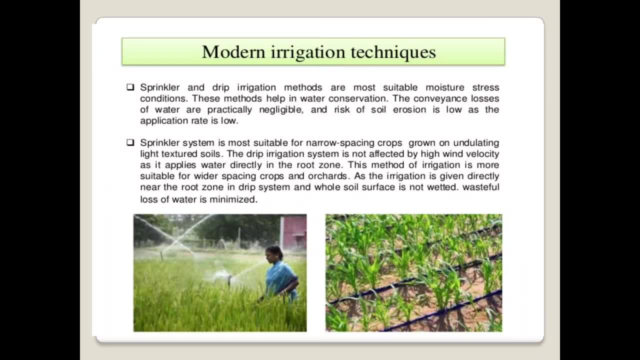 which, having the wide spacing as well as it, is mostly suitable for the orchard. then, as the irrigation which is given directly near to the root zone in the drip system and the whole soil surface is not weighted during the irrigation process, the drip irrigation system is used to 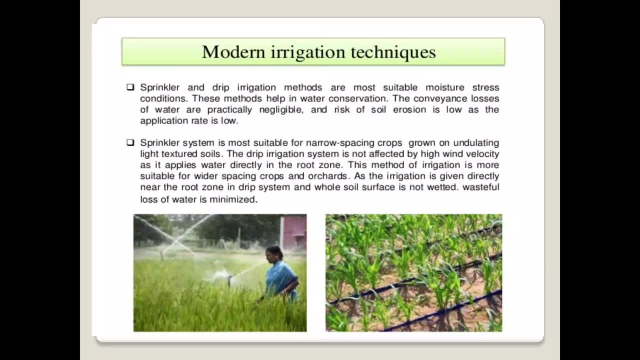 the drip irrigation system. we are applying the irrigation directly into the root zone and due to that the whole surface area of the land that is not wet and the phase losses of water is also minimized. that means the drip irrigation system is very efficient under the rain fed condition. 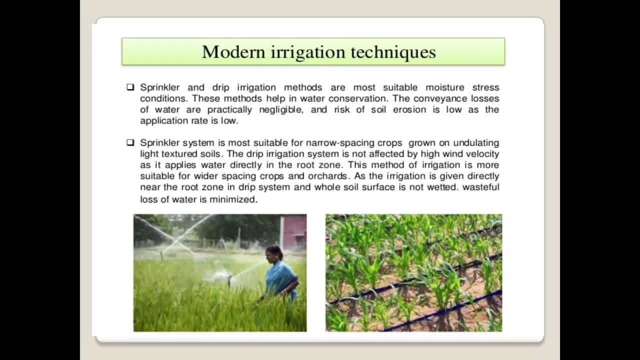 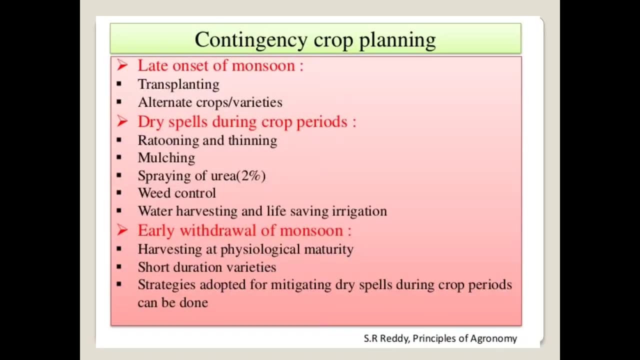 as the application losses of water through this method is very less. then the important practice which is also given to mitigate the drought condition, that is the contingency crop planning. so the contingency crop planning which involves the late onset of monsoon, so in that condition we can adopt the transplanting of the various crop if the onset of monsoon is. 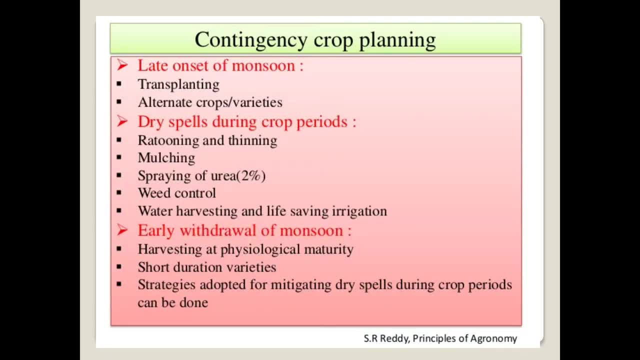 late- that means the late start of monsoon- is there. in that condition, we can plant the crop by the transplanting method. then, in that condition, we can also adopt the alternative, alternate crops or the varieties which, having the short duration as compared to the regular varieties. these important practices which are adopted in case of the late onset of the monsoon. 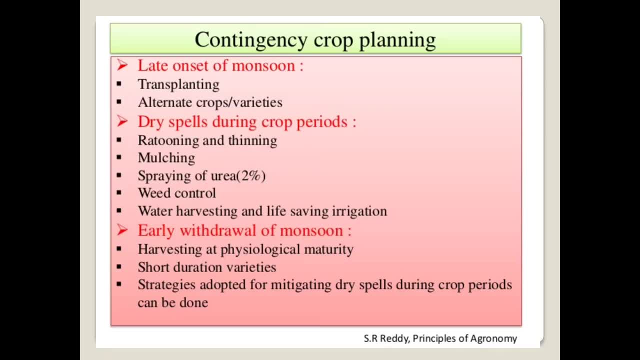 the next one, the dry spell during the crop period. if the dry spell or the stress condition is there during the crop period, then we are applying the returning and the thinning of the crop that means they are helps to minimize the transpiration losses of the plant. then the application of 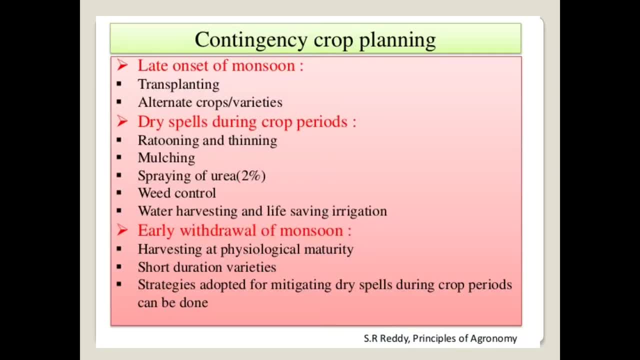 mulches. that helps under the soil moisture, then it also helps to reduces the evaporation and it also helps to maintain the temperature of the soil also. then the important practice which is also followed as the spraying of the urea. that also minimize the stress condition. then timely weed control, which 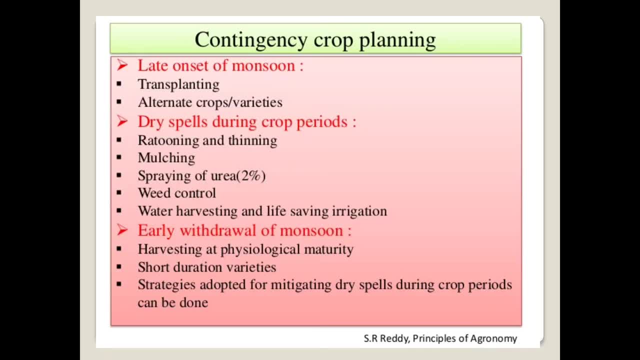 is also essential in the dry spell which is occur during the crop period and due to that, the if the weeds are controlled in time and due to that, the transpiration losses of the transpiration losses is minimized as well as the crop and weed competition is also minimized in that 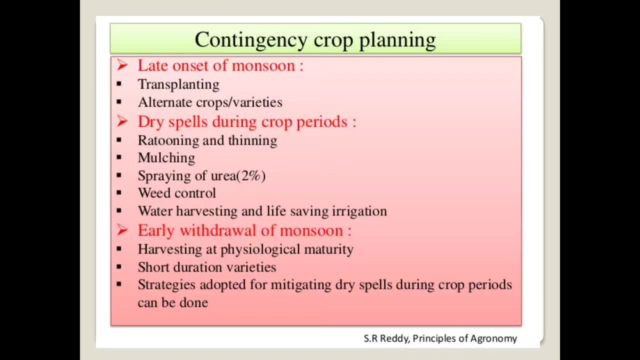 crop plot, then the water harvesting and the life-saving irrigation that also plays the very important role. if the dry spell which is occurred during the crop period, then next one, that is, the early withdrawal of the monsoon. if there is the early withdrawal of monsoon, that means the late, early stop of the rain that takes place during that condition. at that time the 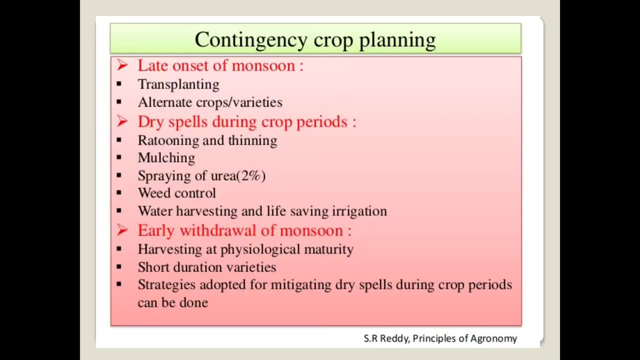 crop, crop at a physiological maturity stage, which is carried out, then the short duration varieties which are selected and they are also harvested early during the early withdrawal of the monsoon. then the strategies adopted for adopted for mitigating the dry spell during the crop period. that can be also done to minimize the moisture stress condition or the drought condition. 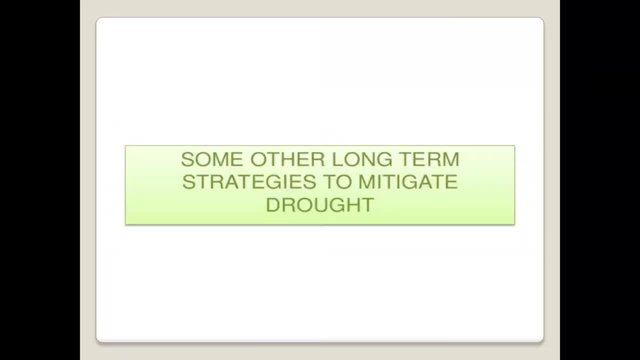 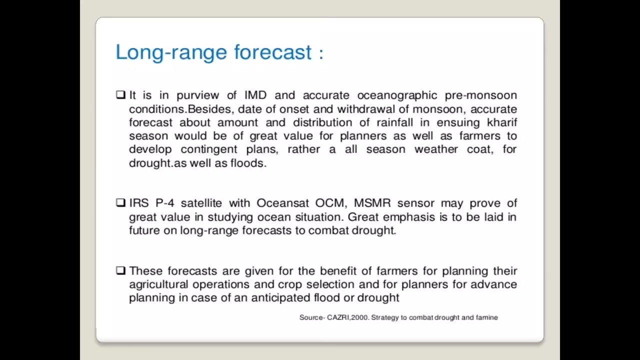 then some other long-term strategies which are also used to mitigate the drought. then, under the long-range forecast, it is in preview of imd and accurate. accurate oceanographic pre-monsoon conditions, besides the date of onset and withdrawal of monsoon, then accurate forecast about the amount. 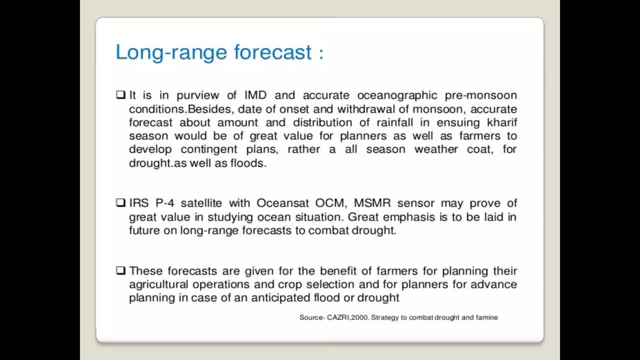 and distribution of rainfall is in during the creep season would be of a great value for the planners as well as the farmers to develop the contingent plant, rather a all season weather code for the drought as well as the flood condition. that means, under the long range forecast, it is always forecasted that the 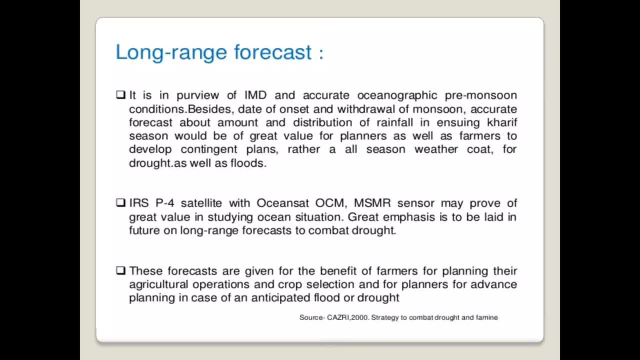 onset as well as the withdrawal of monsoon, and how much amount of thelegt that can be received during a particular year. that is also helps for the planning of the farmer, as well as the other scientistsMean crit èm another fish. other scientists, too, to be. 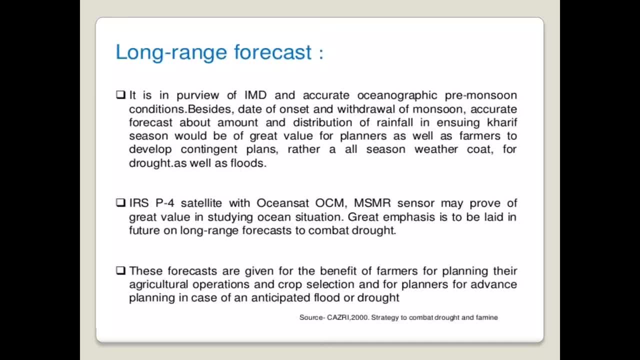 I hope you found this video helpful in real time, sending lots of your comments. Anyway, thank you for doing so much comments on this- farming in a better way and due to that, the drought or the flood condition that is, uh, that can be managed in a better way. so the long-range forecast also plays a very important role in the 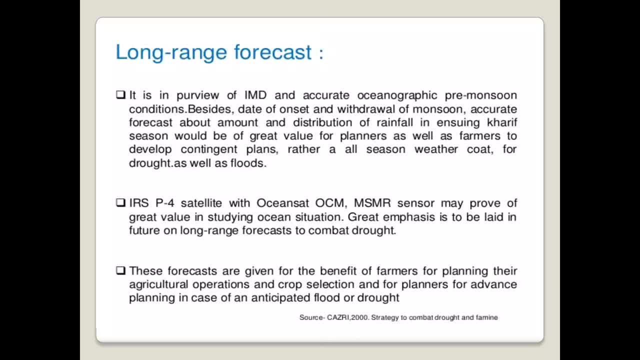 management of the crop under the rain fed condition. then the irs irs4, irs irs p4 satellite with the oceans at ocmr, ocm or msmr sensor may prove of a great value in studying the ocean situation. then the great emphasis is to be led in the future on long-range forecast to combat the 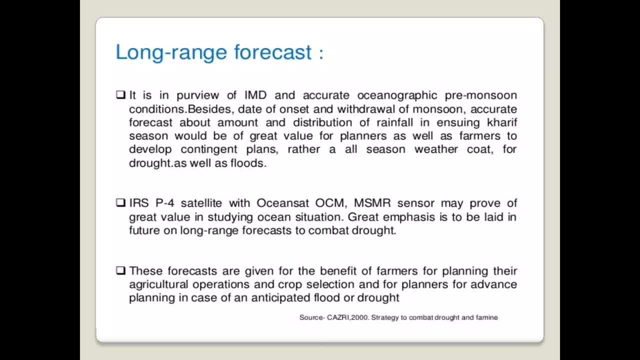 drought condition, then these forecasts which are given for the benefit of farmer, for planning their agricultural operations, as well as the crop selection, and for planners for the advanced planning in case of the agriculture anticipated flood, flood or the drought condition. that means the forecast which is particularly helpful for the farmers, as well as the farmers in planning their various agricultural operations. 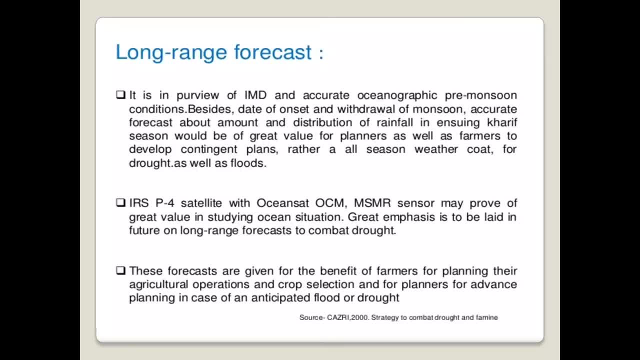 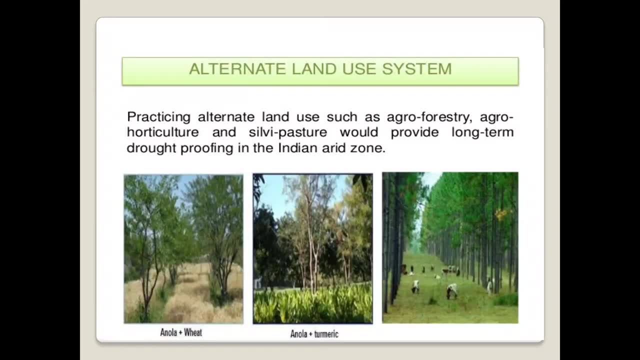 then the selection of crop, and that is also helpful for the advanced planning when the drought condition or the flood condition is forecasted. then the next practice which is used for the mitigation of drought, that is, the alternate land use system. in practicing alternate land use, such as the agroforestry agriculture and silvy pastoral, they have 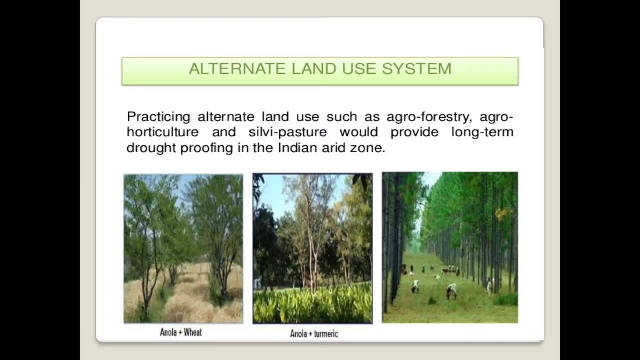 provided the long-term drought proofing. in the indian area zone. that means the alternate land use system that plays very important role in minimization of drought condition as the various crops which are included under that system, as it includes the agronomical crop forestries, then 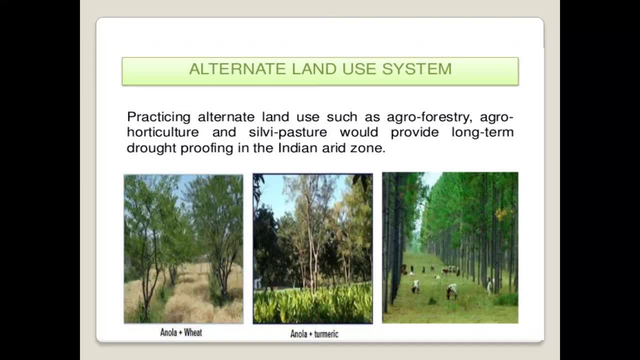 horticultural crops, like some fruit crop, then various grass crops and other crops which are also included under the alternate land use system, for the better management of drought in a rain-fed condition. thank you, they are beneficial. in the indian area zone, for example, there are some cropping systems which are given as a. 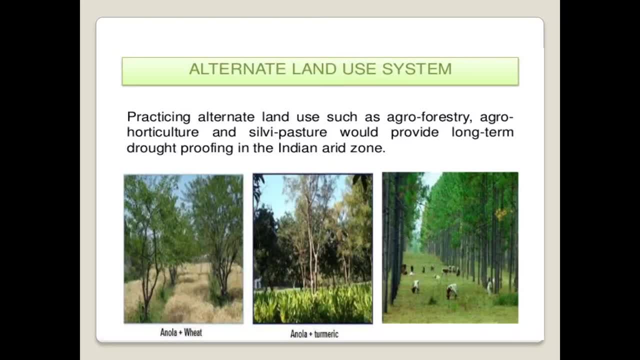 only plus feet, then only plus turmeric. these are the cropping system which are adopted under the alternate land use system for the better management of drought in a rain-fed condition. thank you.